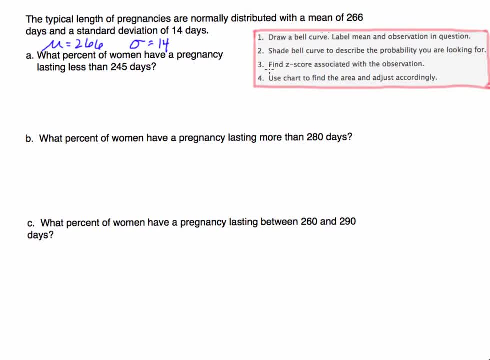 Here's the four steps that I recommend that you follow when you go over these problems. Always, always, draw a picture. Even if you don't follow these exactly the way that they go, I really, really strongly believe that you should draw a picture and including mean and the observation in question. 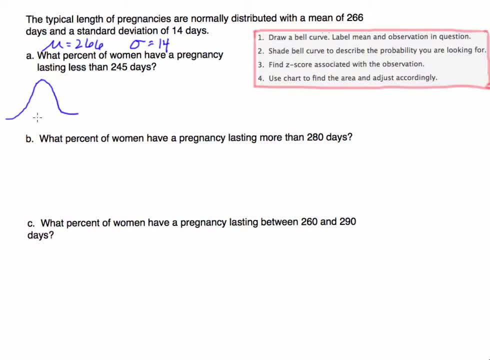 So I'm going to just quickly draw the bell curve and I'm going to label the mean in the middle, so 266.. I will do this for every problem. You'll notice that, And what I'm looking for is I'm looking for in this problem, part A. 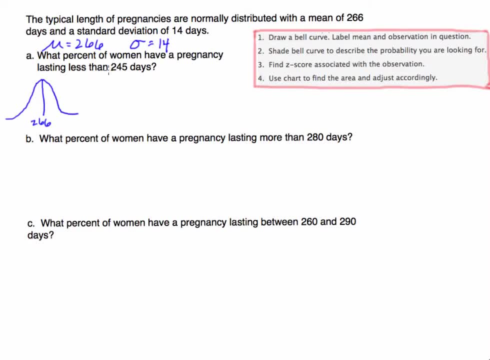 what percent of women have a pregnancy lasting less than 245 days. So here's 266.. 245 would be right here to the left, and I want to know less than that. So I drew the curve, I labeled the mean and here's the observation in question: 245.. 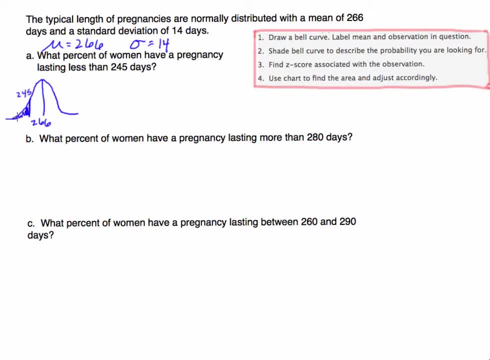 And I want to know the area to the left. So what I need to do? remember that our z-score chart needs a z-score. I need to convert 245 to a z-score. So, if I can take the formula here, I first need to figure out, well, how far away. 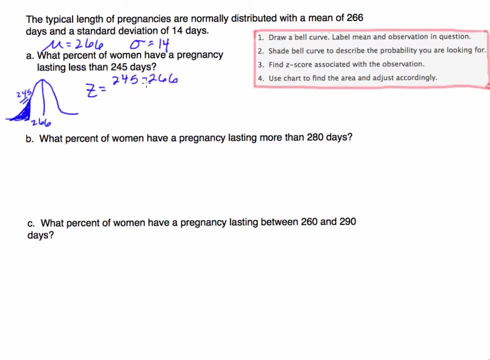 is our observation. and then once I figure out that difference, I'm going to subtract, or subtract them to figure out the difference, and then divide by the standard deviation. So remember, this is x minus mu, all over the standard deviation. So when I plug that into my calculator here, 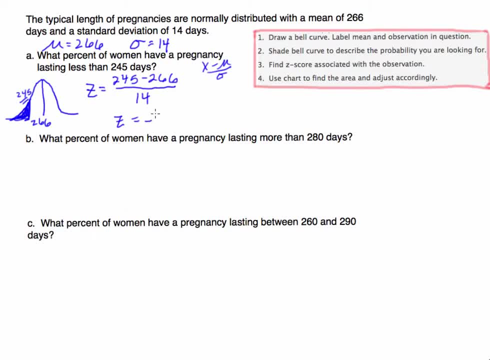 I get negative 1.5.. So what I need to do is to look up the z-score of negative 1.5, on my z-score chart and see what I get. So let's open up the z-score chart. 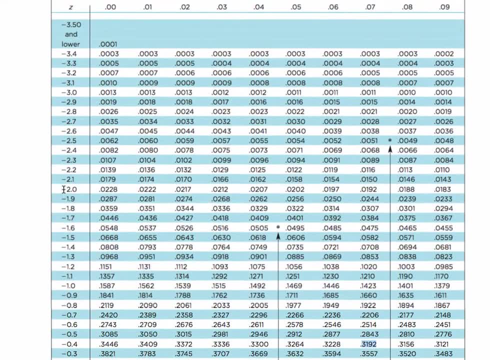 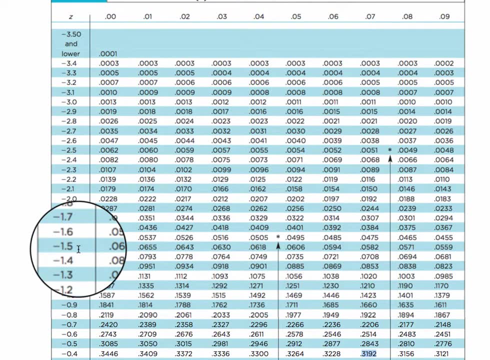 I'm looking up a z-score of negative 1.5.. Here's negative 1.5 right here And I need a 0 in the hundredths column And that is the first column. Notice this is 0, 0.. 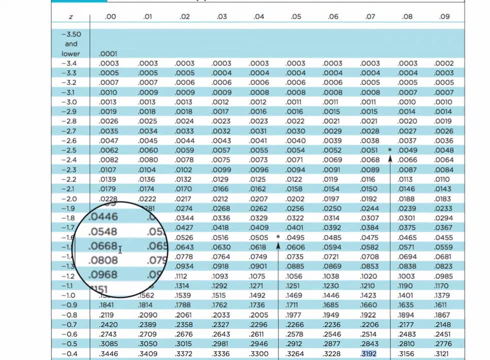 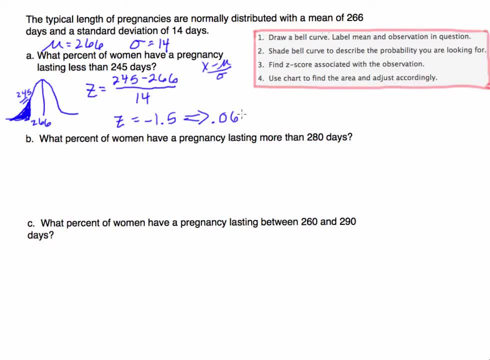 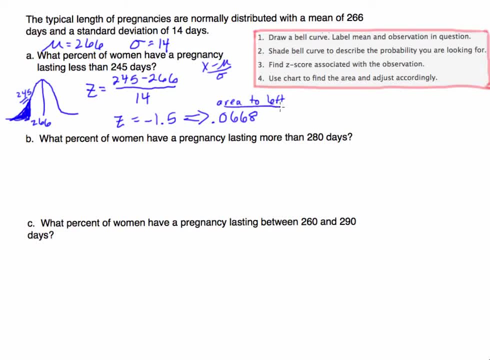 The reason I'm writing this down is because sometimes when you convert z-scores and then you write down areas, you kind of lose track of which is which. Am I talking about an area or a probability, or am I talking about a z-score? 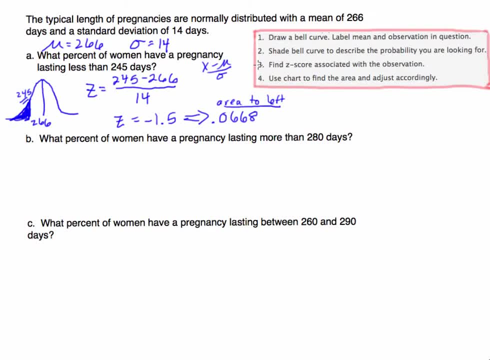 But here this is the area to the left, And now that I've figured out that z-score, I'm going to use the chart to put it in my chart to find the area which I did and adjust accordingly. This adjust accordingly means: is this what I'm looking for? 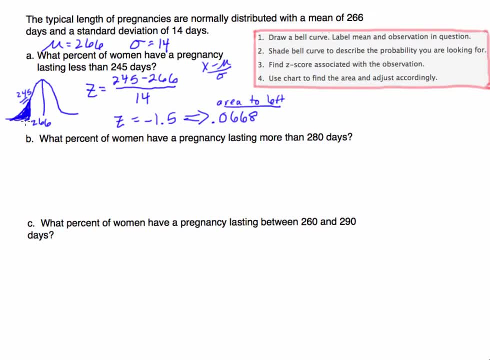 Am I looking for the area to the left of 245?? I am. So what percent of women have a pregnancy lasting less than 245 days? If you convert this probability, this area, to a percent, we get 6.68%. Let's try part B. What percent of women have a pregnancy lasting less than 245 days? Let's try part B. What percent of women have a pregnancy lasting less than 245 days? What percent of women have a pregnancy lasting less than 245 days? 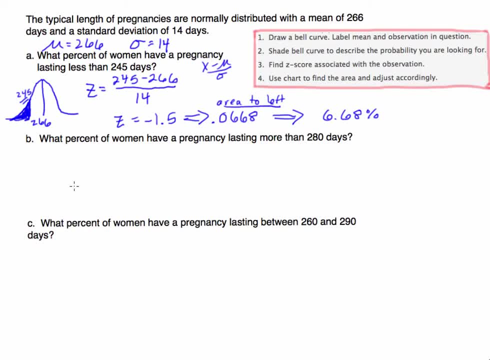 What percent of women have a pregnancy lasting more than 280 days? Always draw a picture. You might get sick of me saying that Here is the mean: 266.. The observation in question is 280, so I'm going to label it 280.. 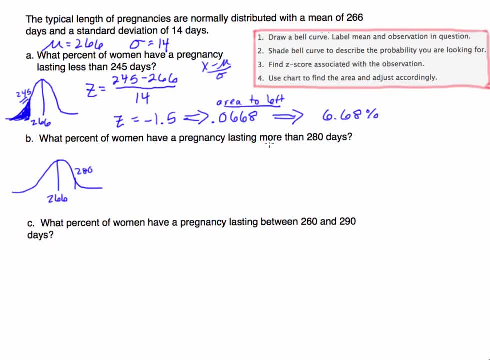 And I'm looking for the percent of women lasting more than 280 days. so I'm going to shade to the right Now. before I find this area, I need to convert 280 to its z-score. So using the formula here, the z-score associated with 280, let's first subtract the mean to. 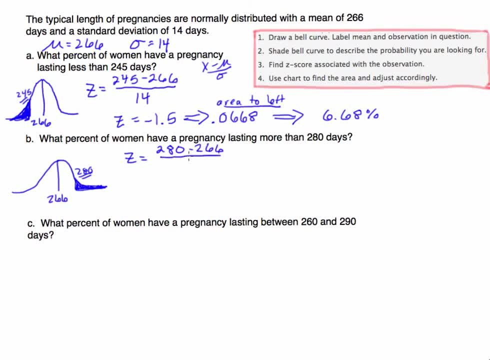 figure out the total distance, And then we're going to divide that by the standard deviation, which is 14.. Divided by 14, I get 1.. We're getting some really nice numbers. I didn't do that on purpose. 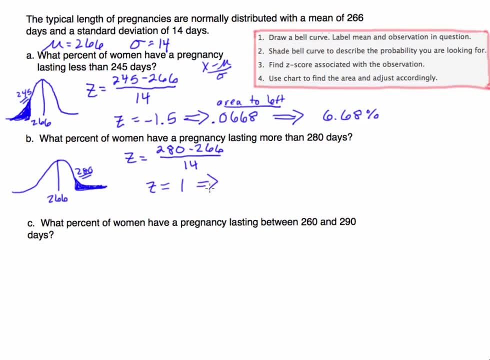 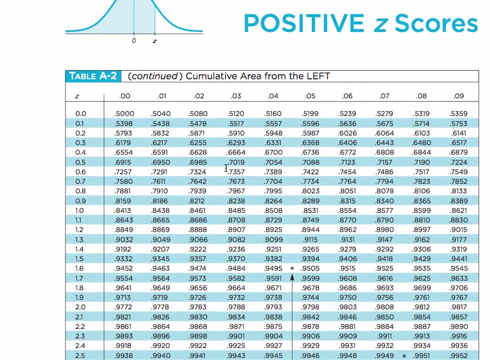 So here we get a z-score of 1.. When I look that up on the chart, let's see what we get. We're going to go to the. here's the negative z-scores. Let's go down to the positive z-scores. 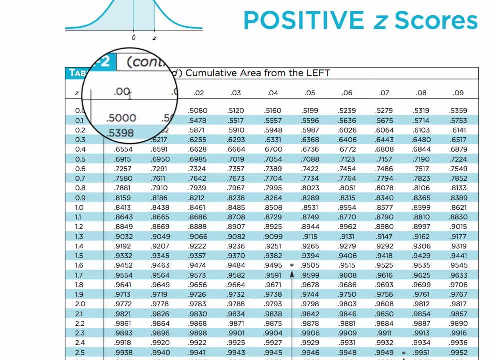 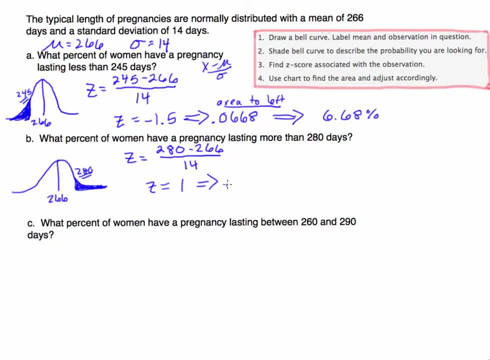 I am looking up here is 1.0, and the column for zeros .8413,, 8413, .8413.. And again, this is the area to the left. Am I done? Usually when I ask that question, the answer is no. 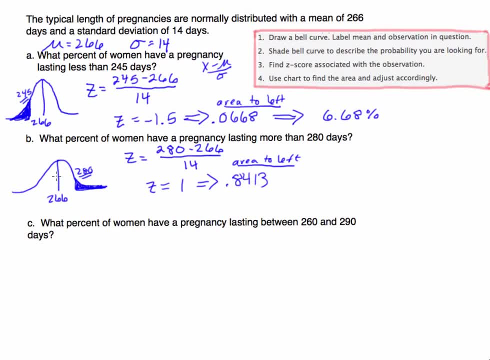 The reason why: .8413,- this is the area to the left of 280, and we know that the mean is 266.. So how do I get the area to the right? How do I get the percentage of women lasting longer than that 280-day mark? 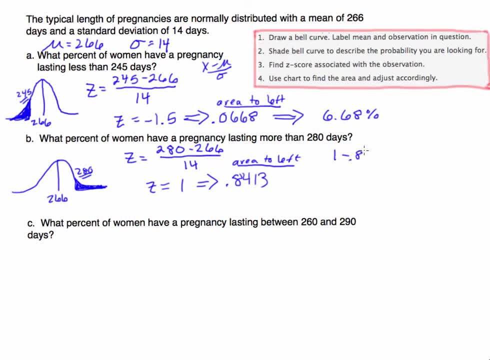 Well, I'm going to subtract .8413 from 1.. Right, We're going to subtract from 1.. The reason why is we want the area to the left Or, excuse me, I want the area to the right. So when I subtract that from 1, I get .1587.. 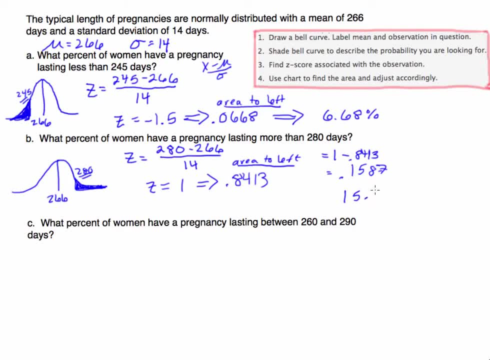 So when I convert that to a percentage, 15.87, and that's a percent In this problem, I still made the picture, labeled the observation shaded to the right- Am I done? calculated the z-score and then, once I got the area to the left, I subtracted from one. 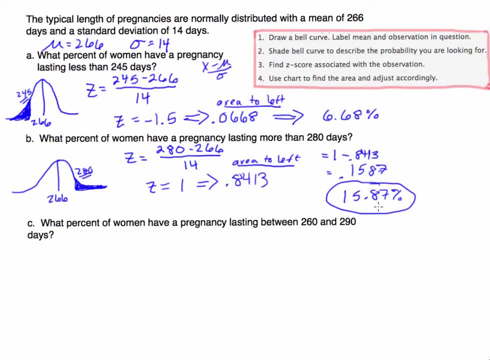 to get the area to the right and converted it to a percent. The final problem says: what percent of women have a pregnancy lasting between 260 and 290?? Well, here's my terrible bell curve. with 266 in the middle, I'm going to label 260 to the left. 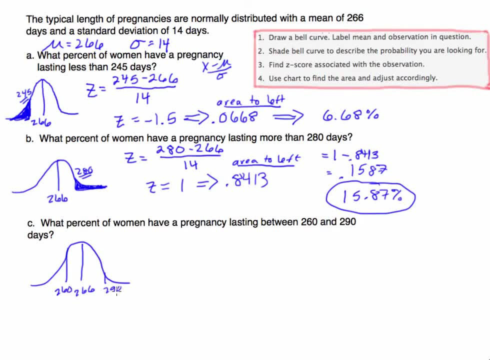 I'm going to label 290 to the right And I'm going to shade in between. This is the area that I'm looking for. I want to know what percent last in between those days. I must find z-scores associated with both of these. 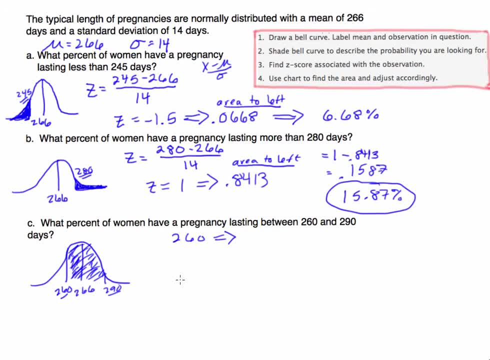 So 260, I need to convert that to a z-score and 290, I need to convert that to a z-score. So there's a little bit more work here. I'm going to let you fill that out. so if you want to pause the video and give that, 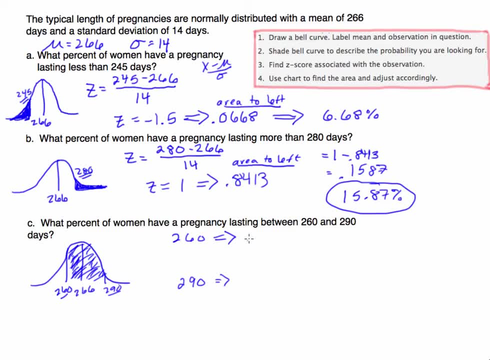 a shot. when you come back and unpause it, the answers will be here. The z-scores will be calculated. I went ahead and calculated the z-scores, rounding them to the hundredths place. Now I'm going to look up these values on the z-score chart. 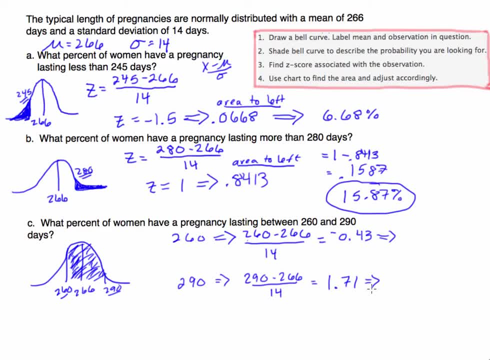 So once again, I'm going to give you the opportunity here to pause the video and try to find the areas associated with both of these z-scores. Okay, So when I looked up negative Negative 0.43,, I get an area to the left of 0.3336.. 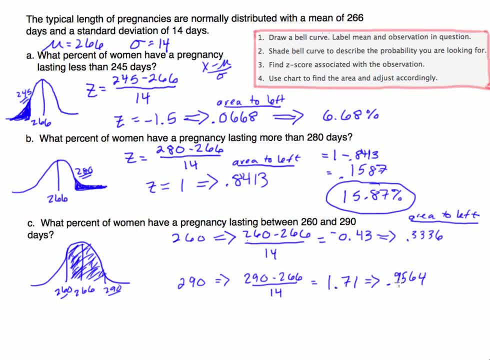 And when I look up positive 1.71, I get an area of 0.9564.. Remember, when I'm looking for the area in between, I need to start with the larger amount and subtract that 260 amount, that smaller amount, so I can get what's in between. 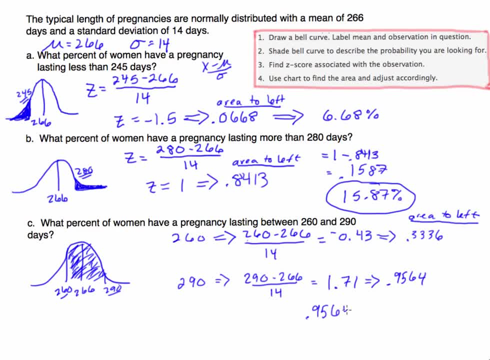 So my final answer will come from subtracting a value: of 0.3336.. From that larger area to the left. So when I subtract 0.9564, excuse me, I take 0.9564, subtract 0.3336, I get 0.6228.. 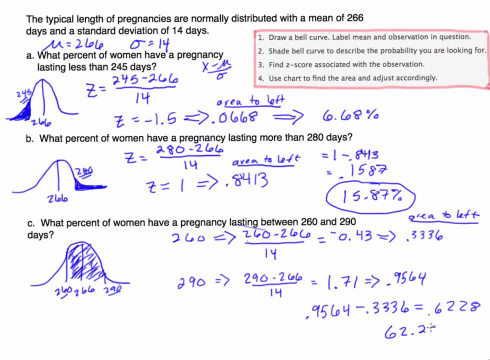 So my percent is 62.28%- And all of these problems on this page. I'm not going to be able to solve them all at the same time And I'm going to start with the area to the left. So in order to solve this problem on this page, it is necessary to first draw a picture. 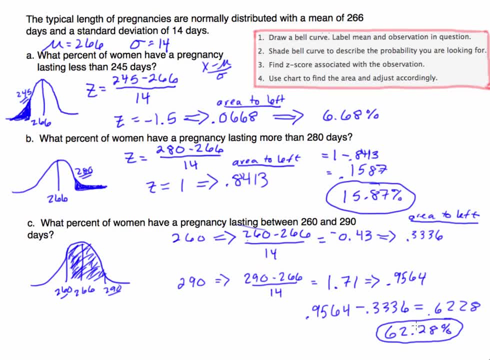 label the observation in question. make sure you shade to the left or to the right or in between, depending on what is being asked of you. We need to then find the z-scores associated with those observations so that we can use the chart to find the area to the left. 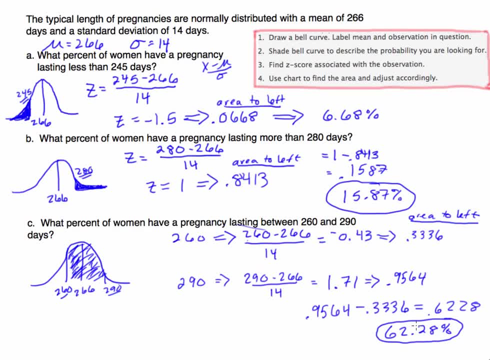 And then if we need the area to the right or we need the area in between, we will subtract from one or subtract multiple areas to find that area in between.